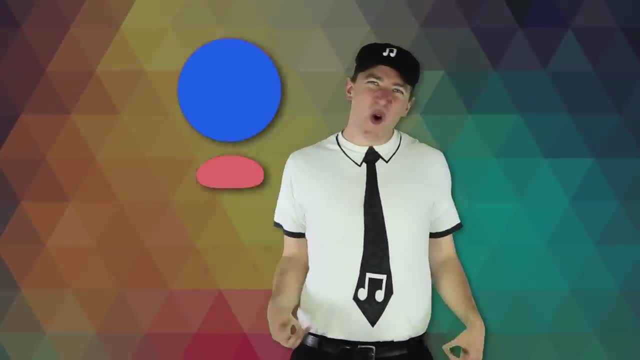 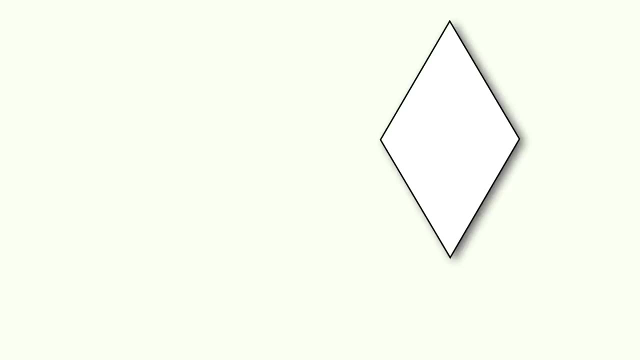 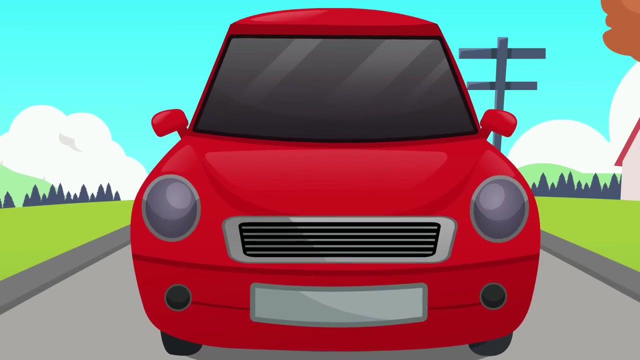 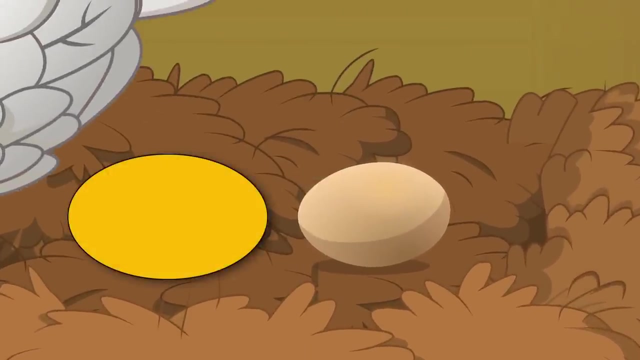 Shapes- Oh my, There's so many shapes, Shapes all around me. Shapes- Oh my, there's so many shapes. Shapes are what shape the world. Stop signs are octagons And chicken eggs are oval, Starfish are star shaped And a kite is a diamond. 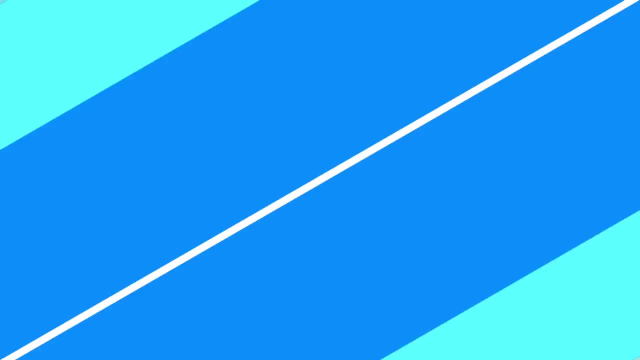 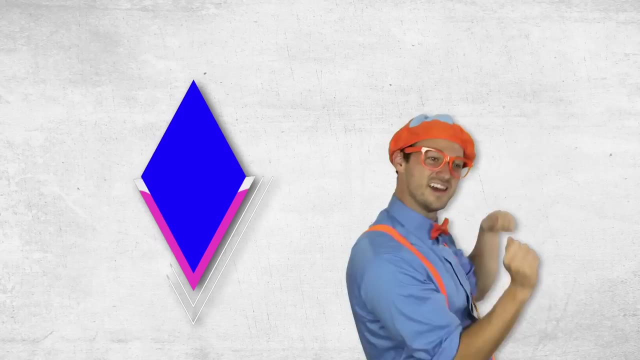 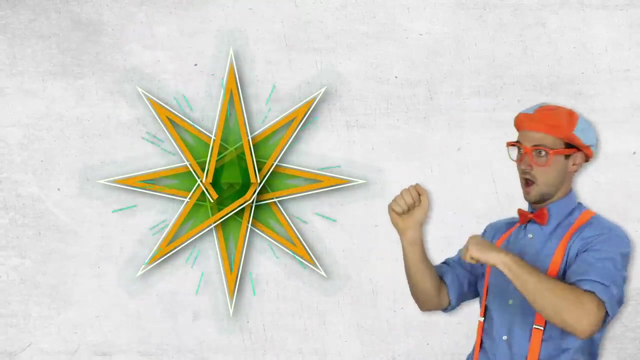 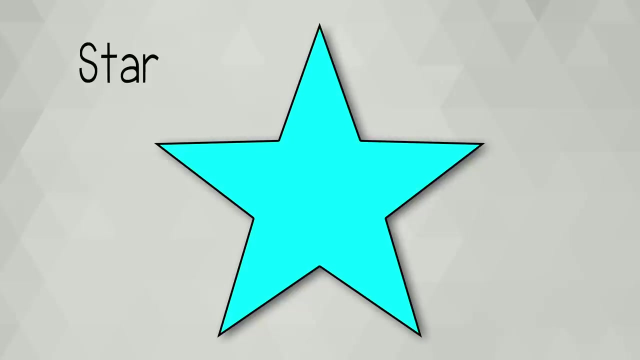 Starfish are star shaped And a kite is a diamond. Starfish are star shaped And a kite is a diamond. Octagon- oval star diamond. Octagon oval star. diamond Square, circle, triangle, rectangle. octagon Star oval, trapezoid diamond, pentagon. 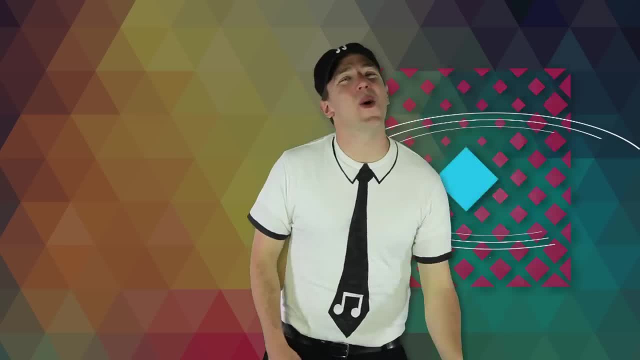 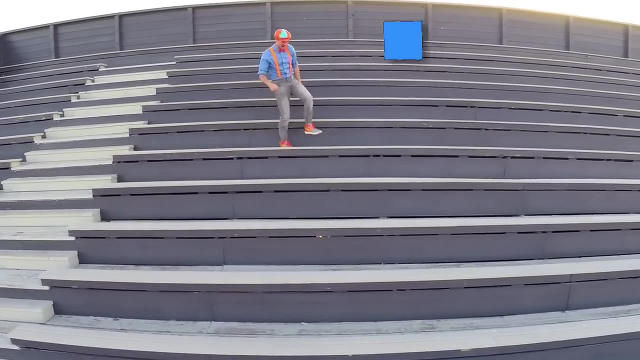 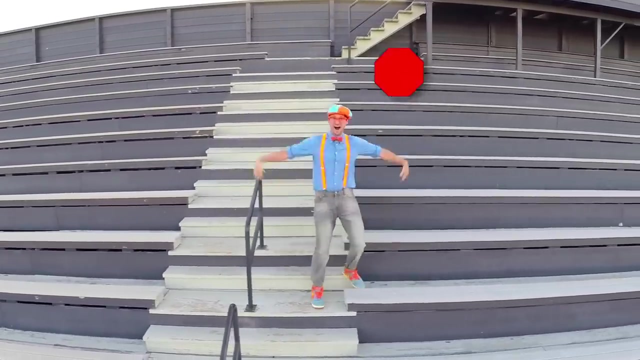 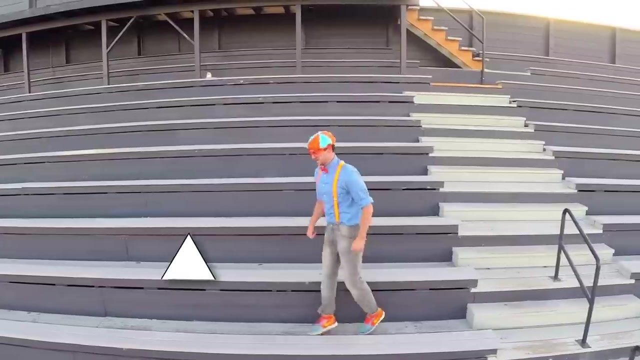 Shapes- oh my, there's so many shapes, Shapes all around me. Shapes- oh my, there's so many shapes. Shapes are what shape the world. Shapes- oh my, there's so many shapes, Shapes all around me. Shapes- oh my, there's so many shapes. 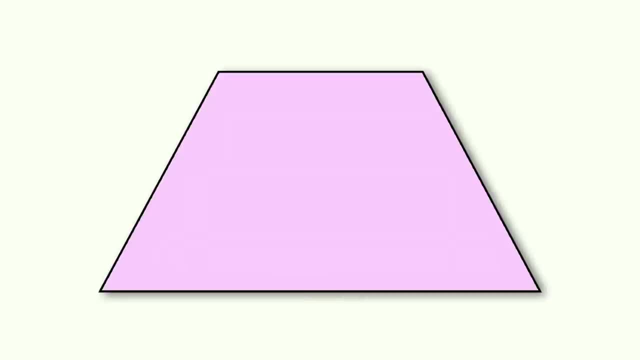 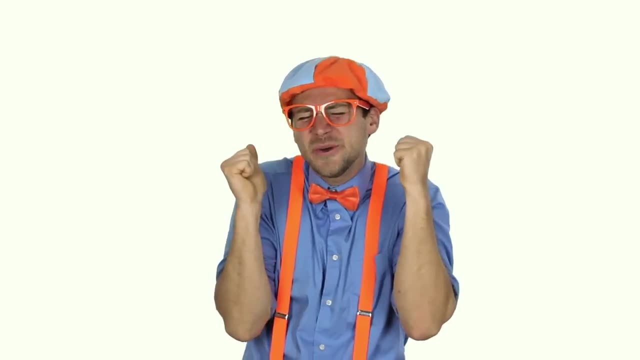 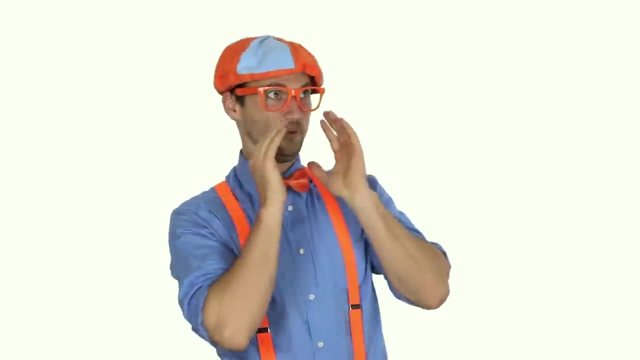 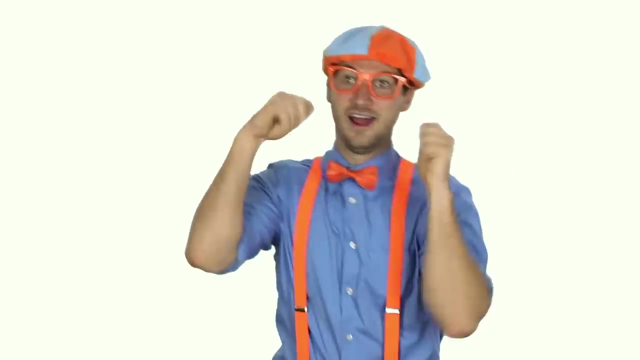 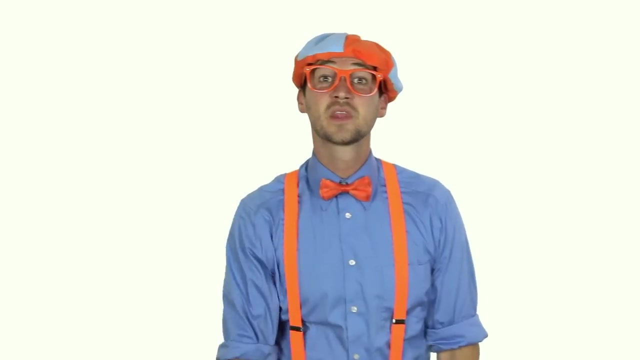 Shapes are what shape the world. That was so much fun singing, Dancing Shapes- oh my, there's so many shapes. Shapes To the shape song with you. If you want to watch more of my videos, you know what to do. Yep, just search for my name. 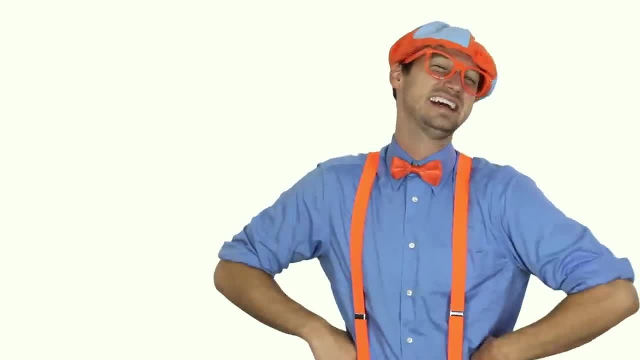 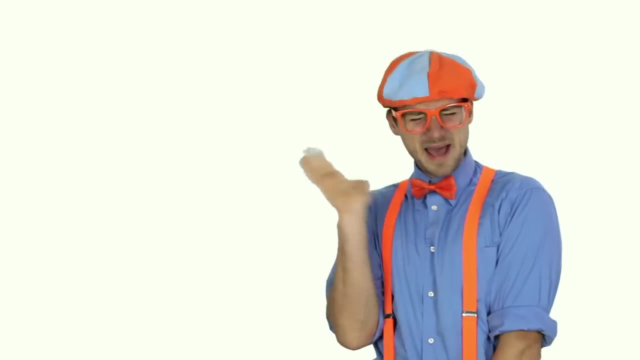 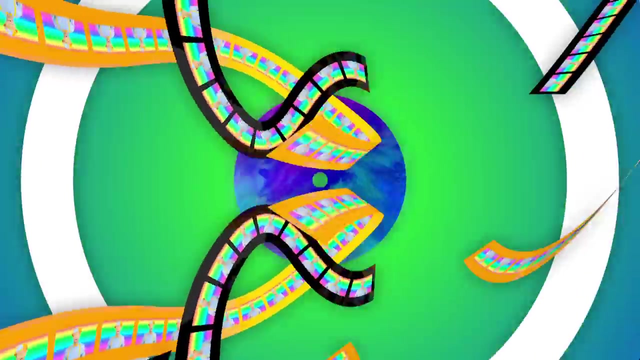